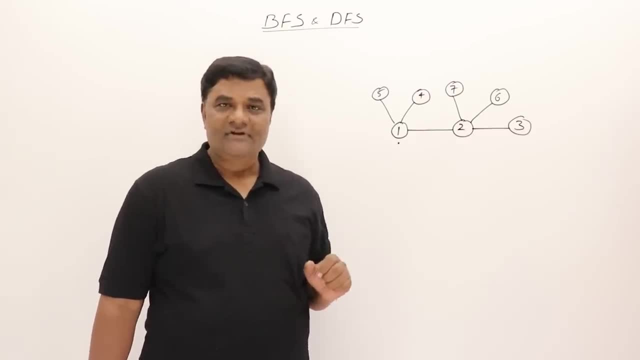 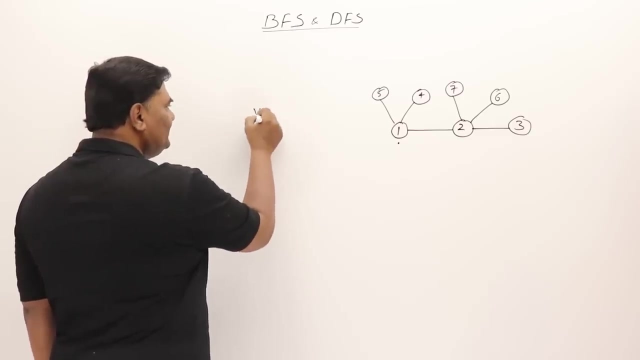 take another example and I will explain you in detail. Now for quick understanding. I have taken a simple graph. Actually, it is a tree, but a tree is also a graph. So let us see. So for traversal- both of these traversal- we have to know these two terms. Now for understanding these traversals, we should know two terms. 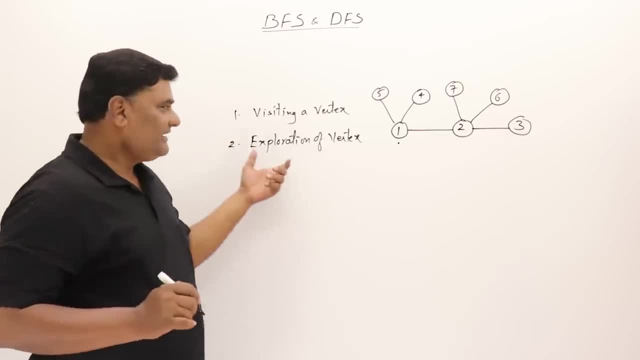 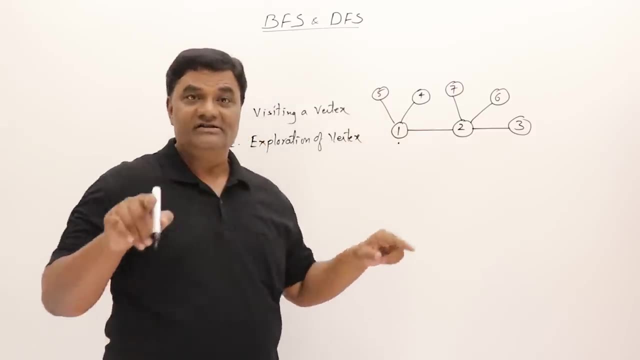 One is visiting a vertex means going on a particular vertex. Second term is exploration of vertex. Exploration means if I am on some particular vertex, then visiting all its adjacent vertices. So based on these two terms we can understand traversals. So first I will explain you. breadth-first search: See I am selecting vertex 1 as the. 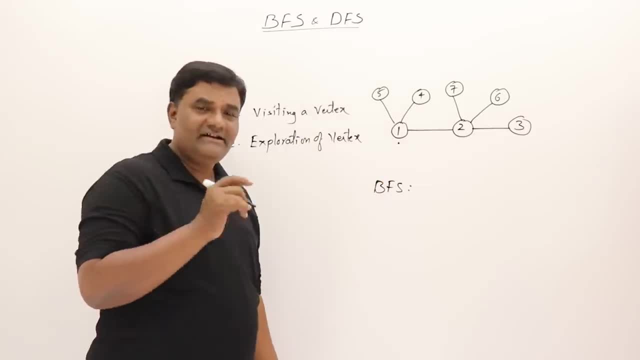 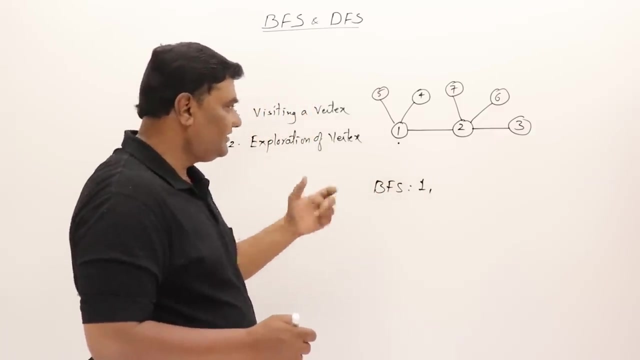 starting vertex to find out. breadth-first search, You can select any vertex as a starting vertex. Now vertex 1,. I will visit the vertex 1.. Now, once the vertex is visited, this vertex I will start exploring means I will visit all adjacent vertices. So who are those For? 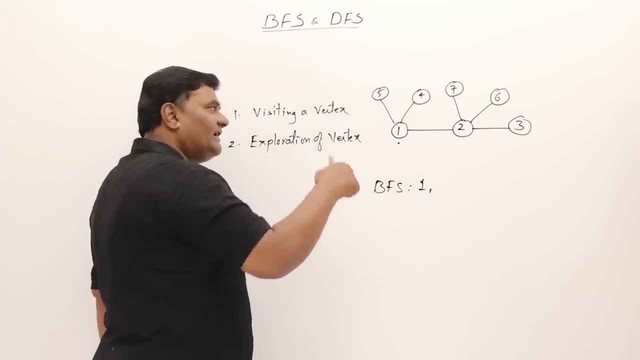 example, 5, 4 and 2.. In which order I can visit? I can visit them in any order. So okay, I will take 2 first, then 4, then 5.. Next I should select the next vertex for exploration. So these are already visited vertices After. 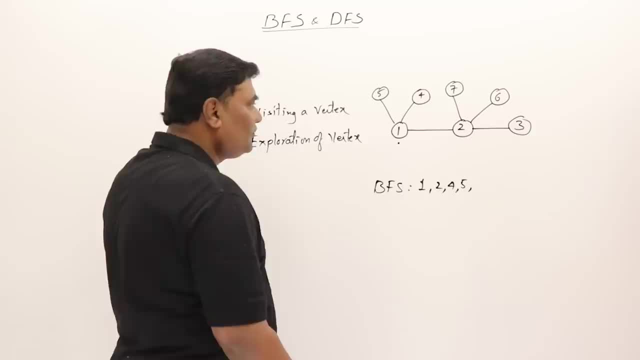 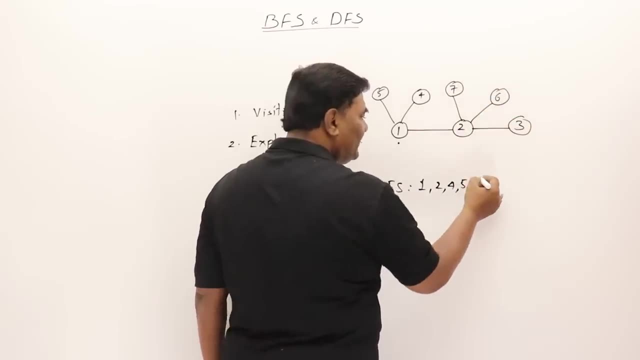 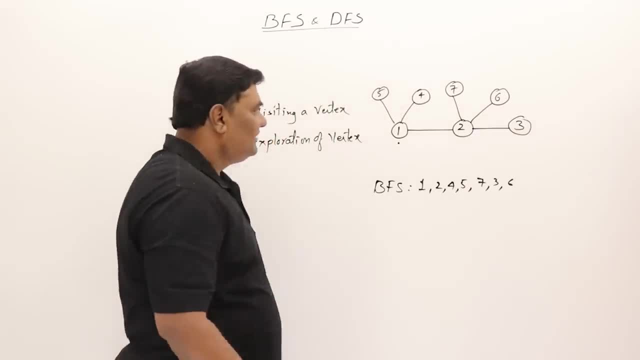 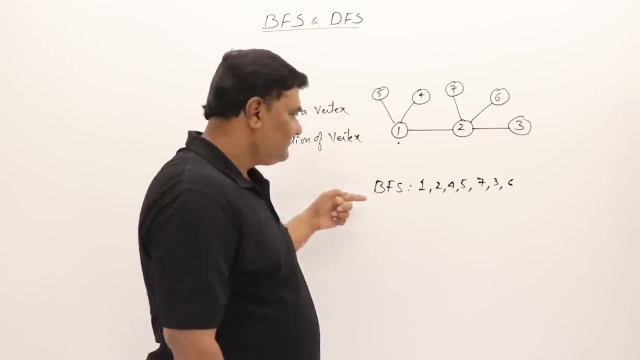 7, 7,, 7, 7, then 3, then 6.. In any order you can take, That's all. All the vertices are visited and there is no vertex remaining for exploration. This is breadth first search. 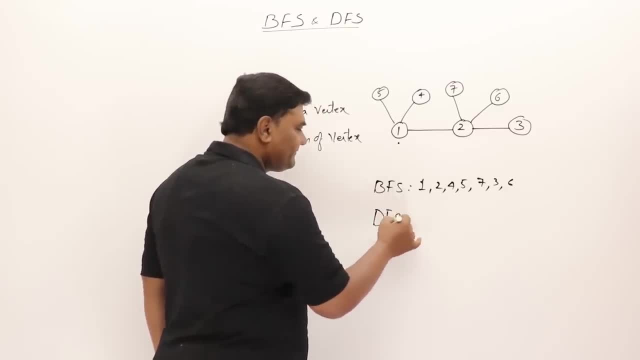 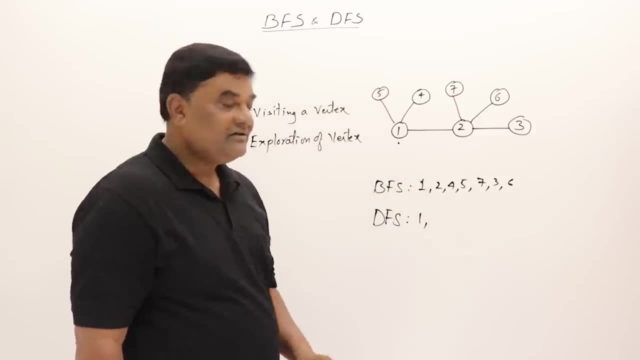 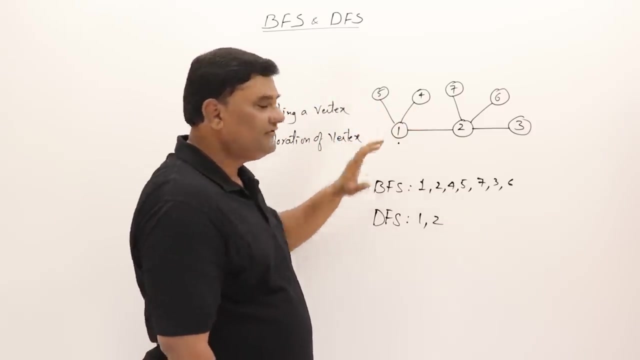 Now let us look at depth. first search: I will start from vertex 1.. Then from 1,. I have started exploration, So I will go to vertex 2.. Now who are other adjacent vertices? Four and five? no, don't visit them. you have reached a new vertex, so you start. 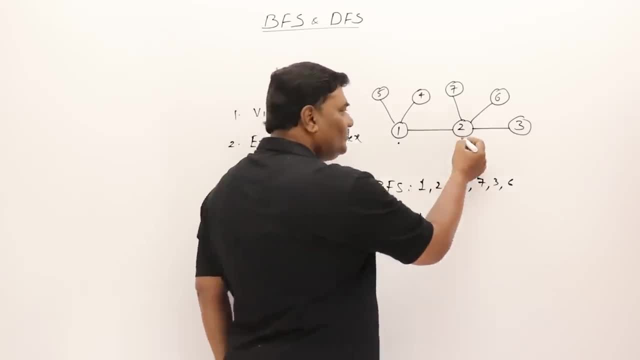 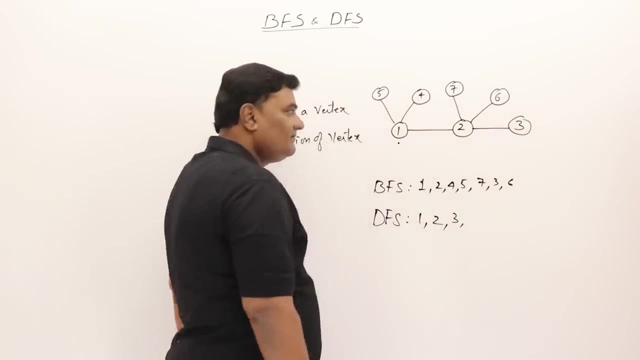 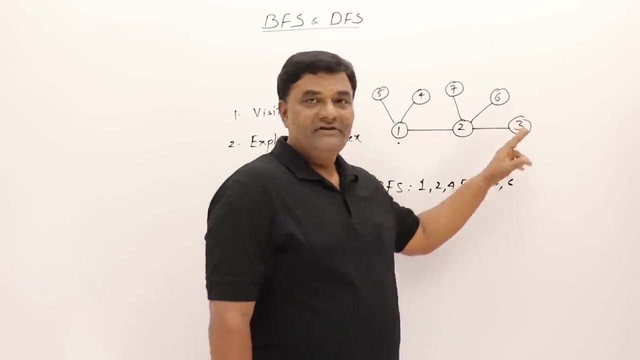 exploring that vertex? okay, I'll start exploring two. then who are adjacent to this? seven, six and three. so I want to go to three. okay, go to three then. shall I visit six and seven also? no, this is depth first search. start exploring three. so if I start exploring three, there is nothing connected to three. okay, so it. 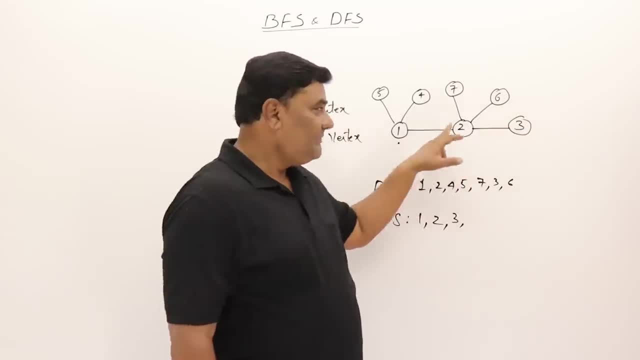 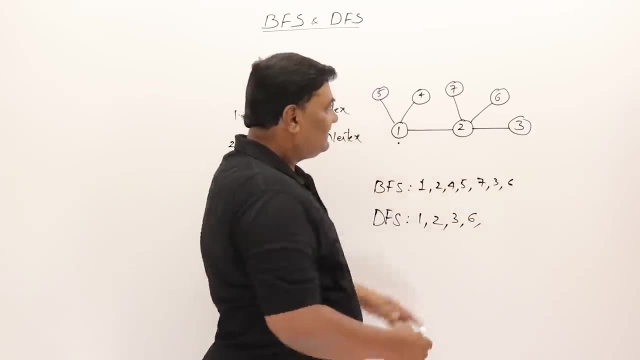 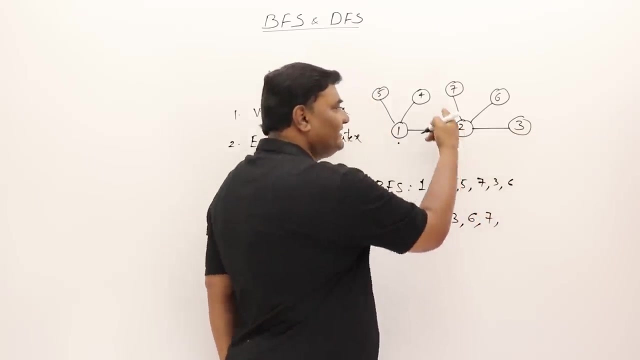 means three is completely explored. then come back and then continue the exploration of two. so who are there? six explore six. nothing is there. come back, go to seven, explore seven. visit seven, explore seven. there is nothing. so come back to one now and continue the exploration of one. who are adjacent to 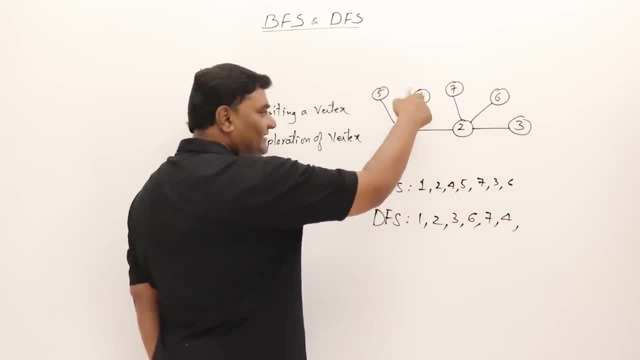 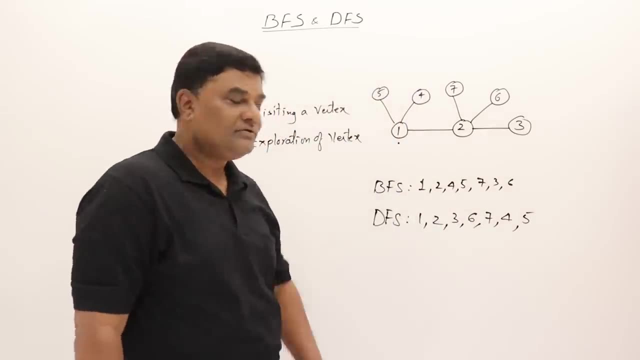 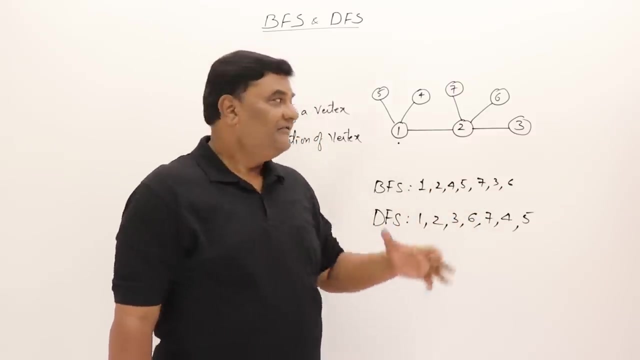 it four, visit four and explore four. there is nothing. come back then go to five, five now. in this way all are explored. so the traversals are different, results are different. so in breadth first search, we will explore a vertex, then we go to the next vertex for exploration. but in depth, first search once we have started. 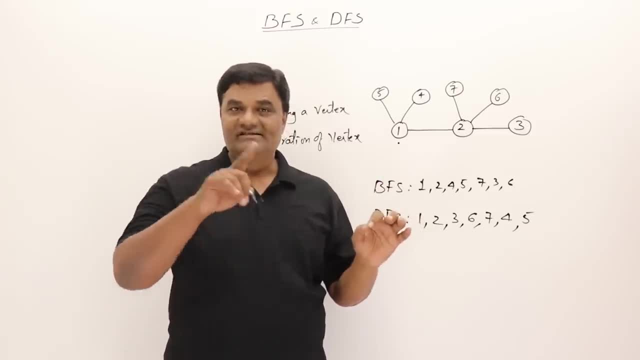 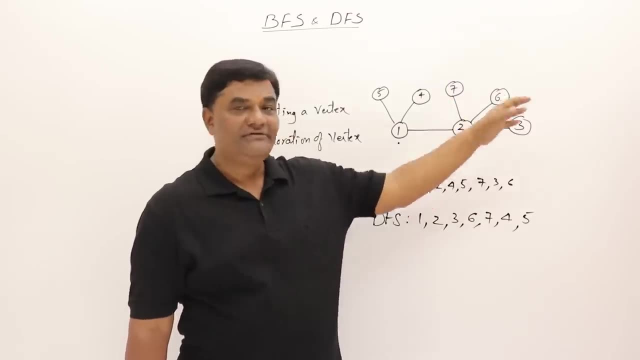 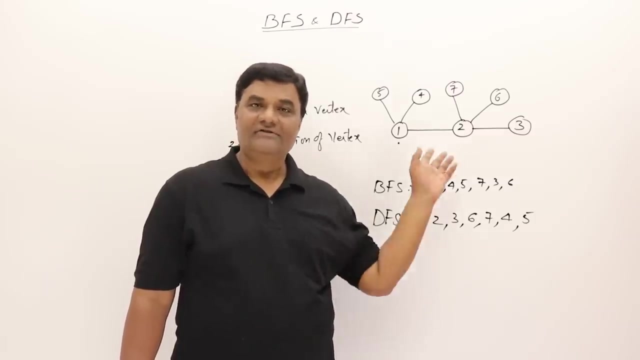 exploring. once we visited a new vertex, we will suspend this vertex and start its exploration. so from one we got two, so we started exploring two, then from two to three and we will start exploring three, like this. so in depth, first search approach is different and breadth for search approach is different. so I will take one more example and 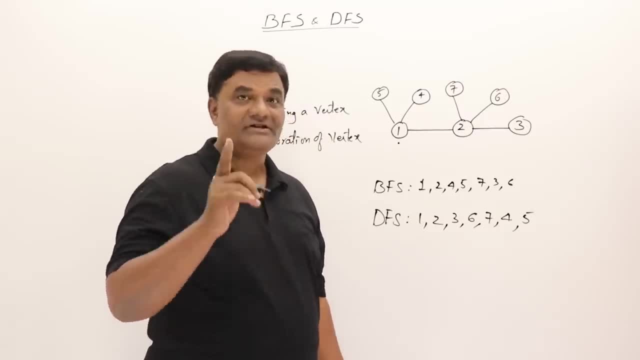 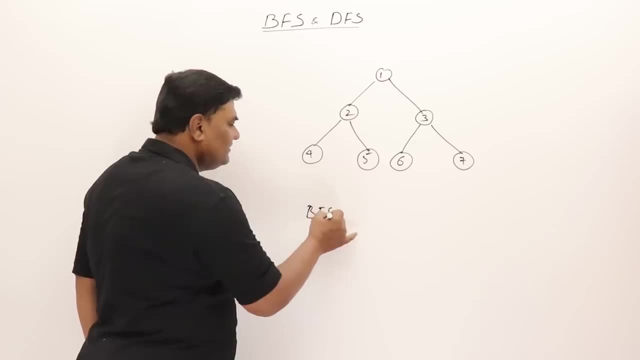 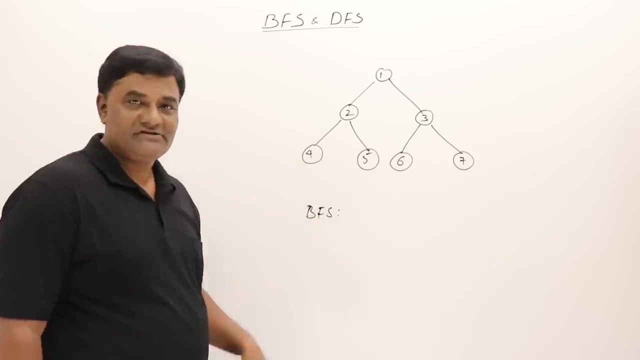 explain you what is the difference between breadth first search and depth first search with a simple example. one more example: let us find breadth first search. actually, this is a binary tree. tree is also a graph. so let us perform breadth first search and see so as per binary. 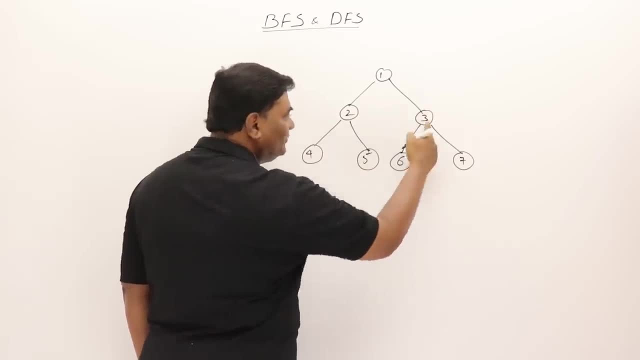 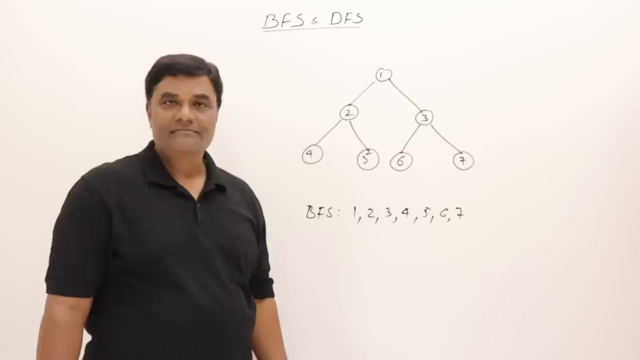 I will perform level order: 1, then 2, 3, then 4, 5, 6, 7, 4, 5, 6, 7. this is breadth-first search, means breadth-first search is just like a level order on a binary tree. then what is a depth-first search? 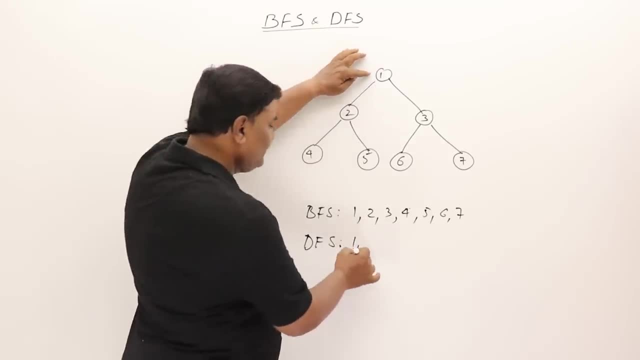 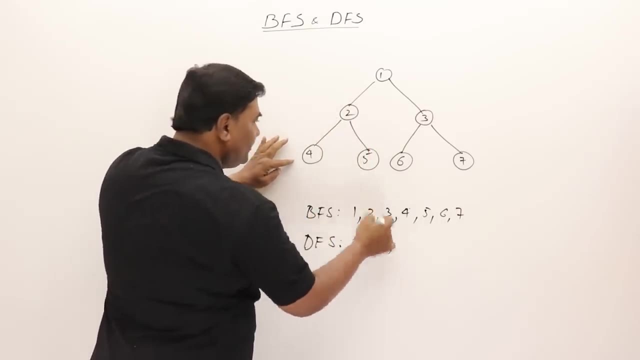 visit 1. okay, explore 1, so we got 2. so stop exploring 1 and start exploring 2, so 4. stop exploring 2 and continue exploration of 4. there is nothing, so go back and come to 5. now nothing is remaining, so go back to 1 and come on this side. 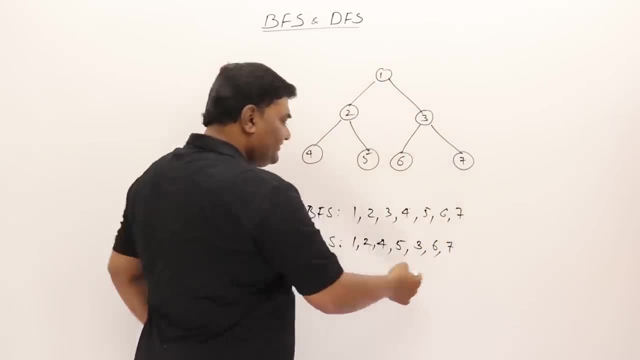 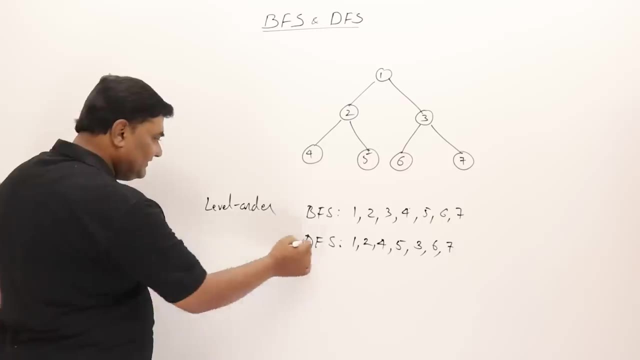 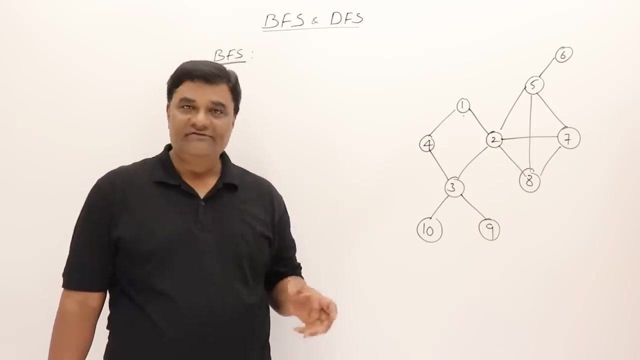 then 6, then go back and 7, so this is like pre-order. so breadth-first search is just like level order and depth first search is just like pre-order traversal of a graph. I have taken a bigger graph now we will learn about breadth first, search and depth first. 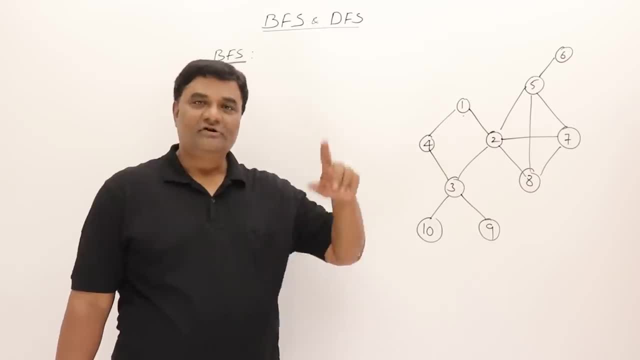 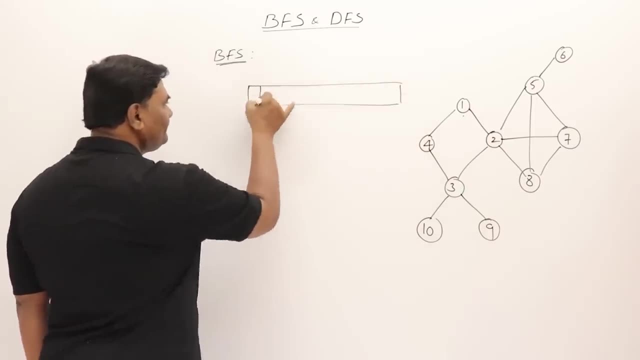 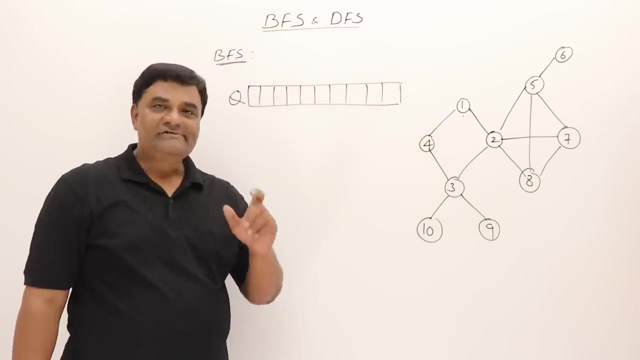 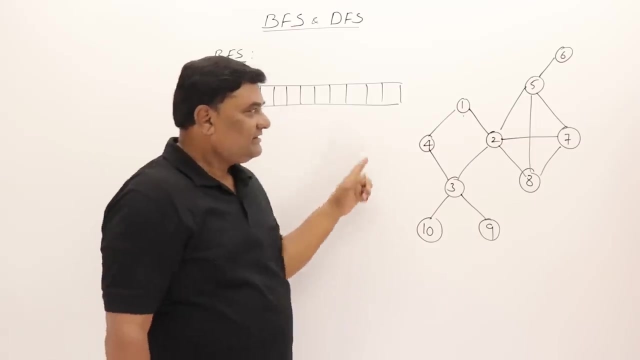 search in detail. first of all, breadth first search. for performing breadth first search, I will take one data structure, that is Q. I have taken a Q. now I'll explain you initial step, then I will explain you repeating step. so what is the initial step? start exploration from any one of the vertex. so which vertex I? 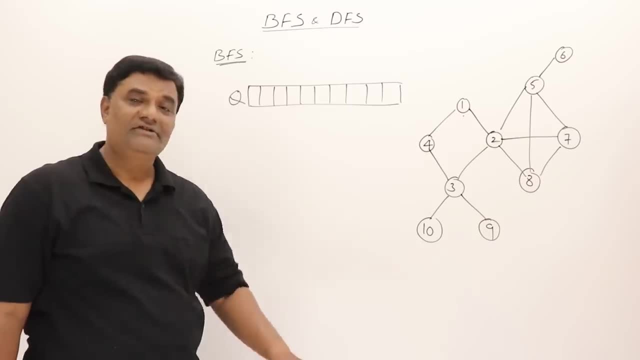 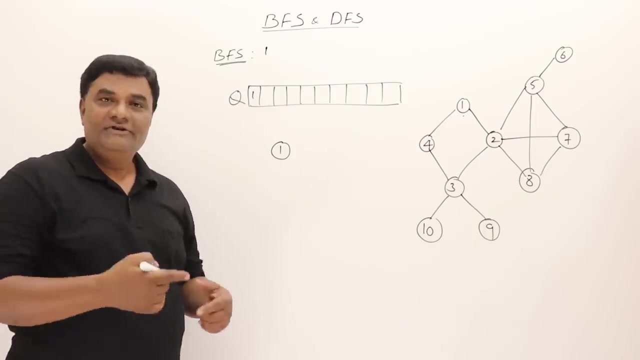 should select as a starting vertex for breadth, first search. you can select any vertex you like, so I'll select vertex one. so in the answer you show it one in the graph you draw here again, then add it to Q. this is the first step, initial step. now we will perform repeating steps. so what are those? 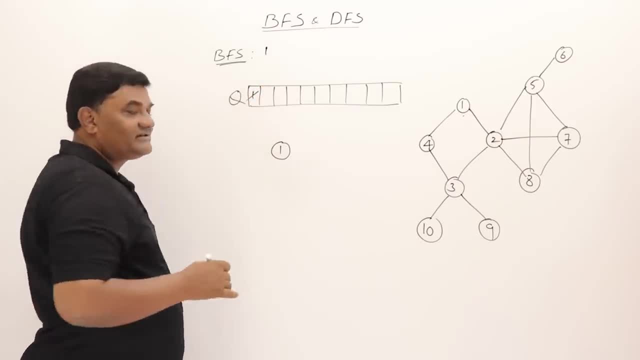 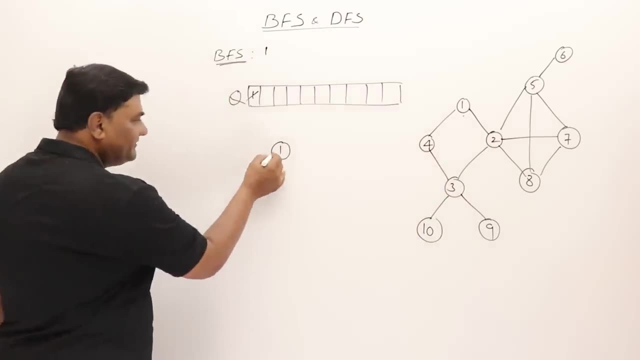 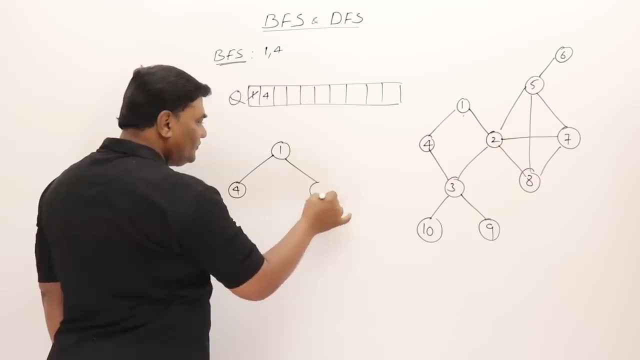 repeating steps. take out a vertex from Q and start exploring it. so vertex one: who are adjacent to one, four and two. so explore them. so first I want to visit four. okay, add it to result and also add it to Q. next I want to go to two. okay, 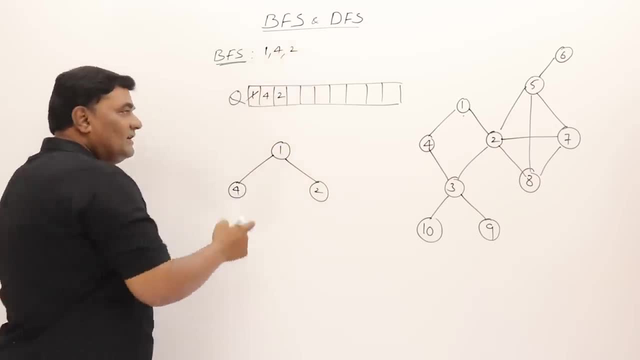 okay, so I want to go to Q next. I want to go to Q next. I want to go to Q next. okay, so I want to go to Q next. I want to go to Q next. I want to go to Q next. add it to result and also add it to Q. now one is completely explored. there is 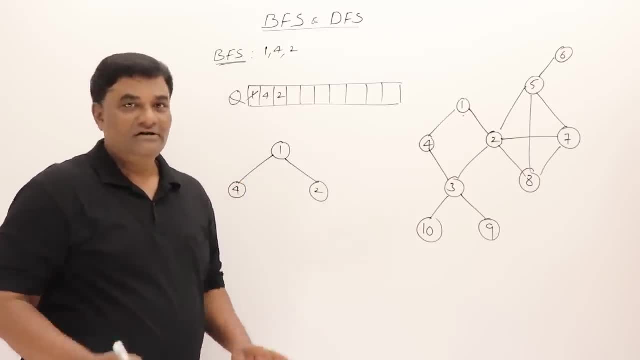 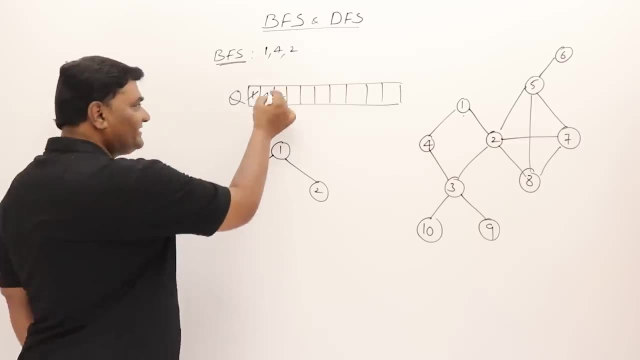 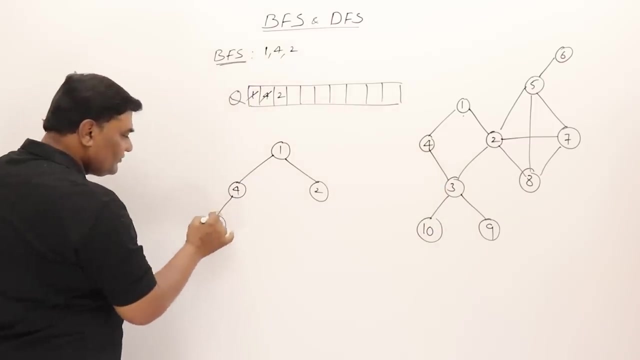 no adjacent vertex remaining for vertex one. this is first iteration completed. now repeat the procedure. what to do next? select next vertex for exploration from Q, that is four. start exploring four. so who is adjacent to four? three, so I'm drawing it like a tree here. so three is adjacent, so add it to Q. any other adjacent for? 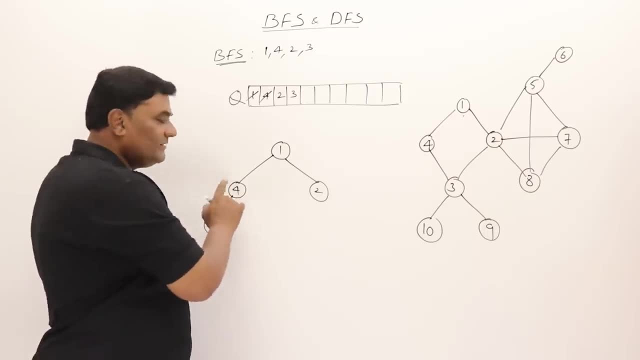 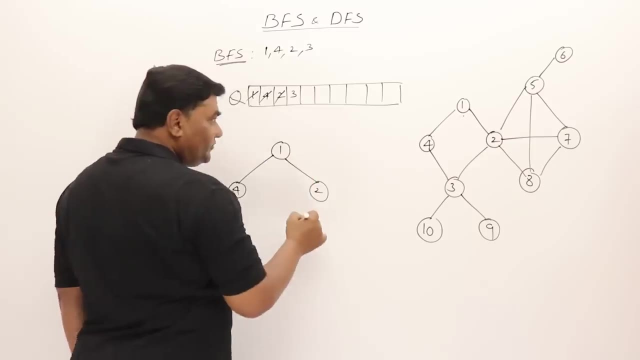 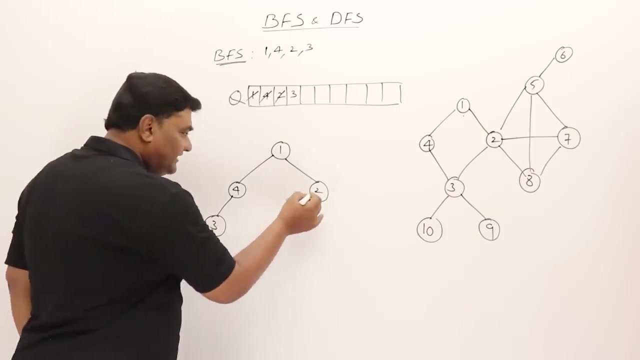 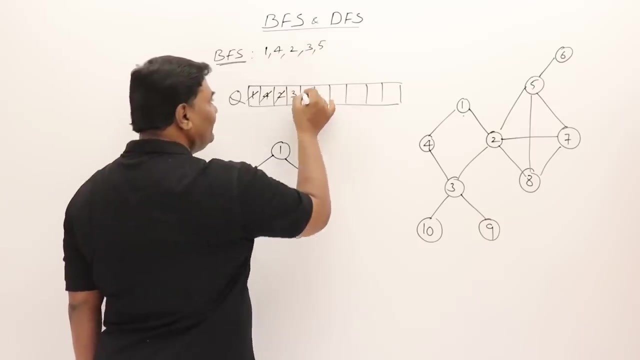 four. nothing is adjacent for four, so four is completely explored. now select next vertex for exploration. that is two who are adjacent to two: three, five, seven, eight. I can visit them in any order. if I check, three it's already explored, so then I will prefer going on five first. so five, five next. I want to go on eight, okay. 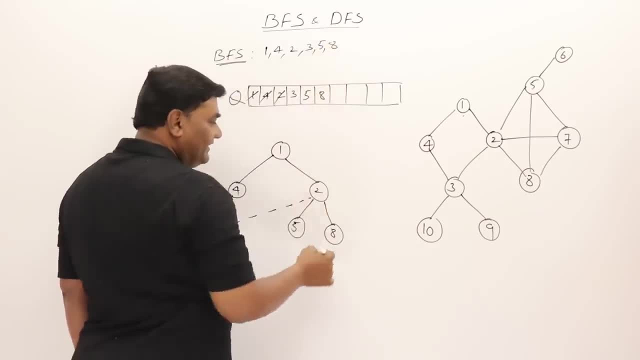 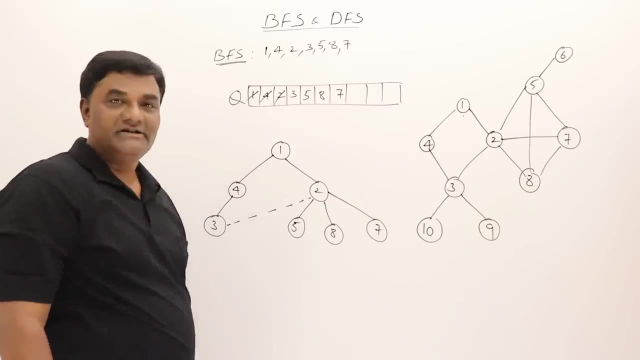 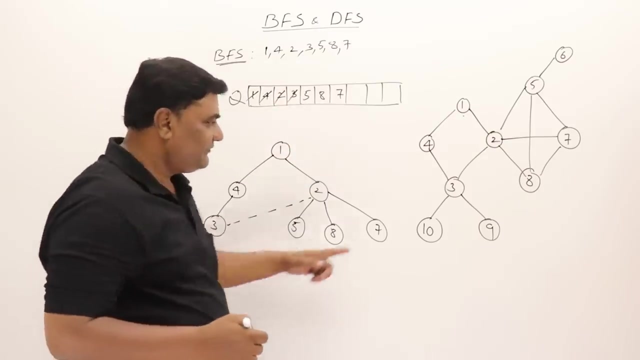 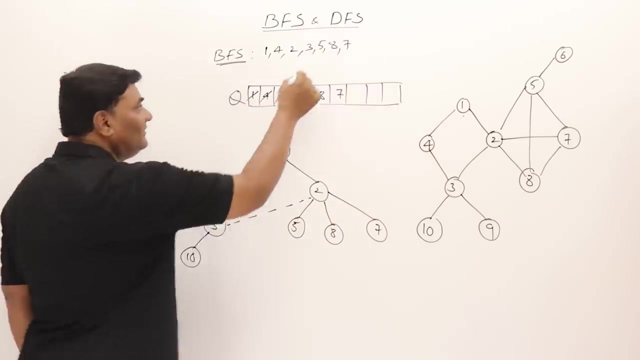 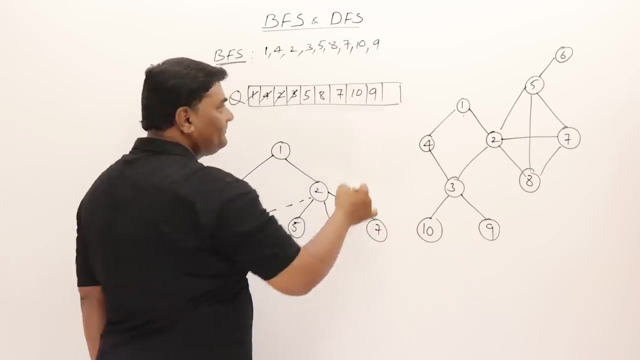 eight, so eight and eight. next I will go on seven, so seven and add seven here. now two is completely explored. now select next vertex for exploration. who is that? three, is there any adjacent vertices for three? yes, two, eight, nine and ten. so two is already visited. so first I will take ten, ten, ten and then nine, nine. add it to Q. 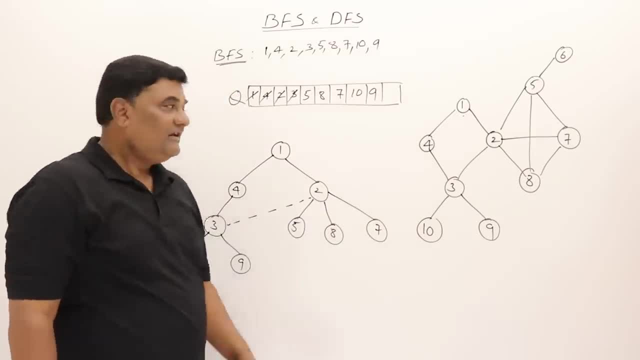 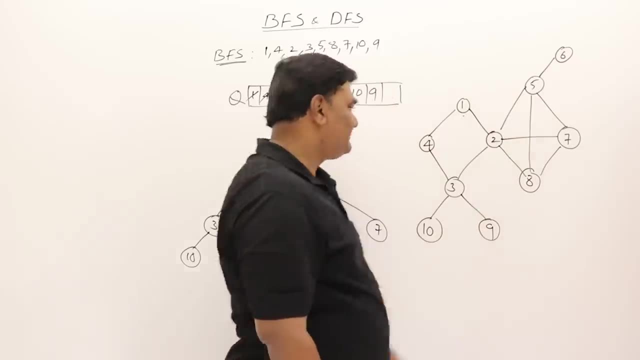 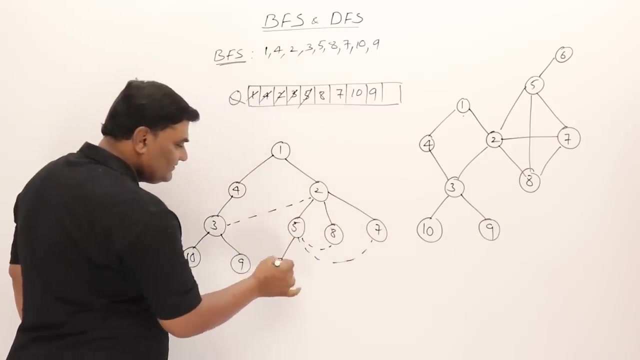 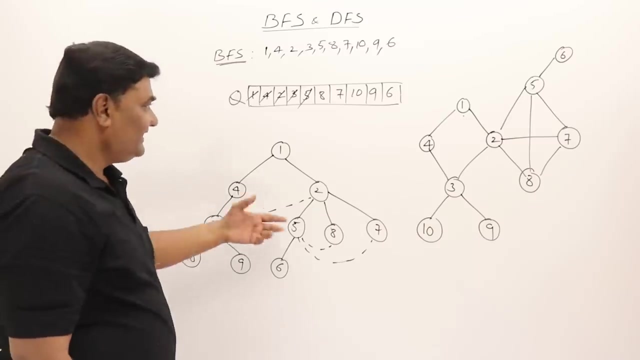 completed. three is completely explored. now select next vertex for exploration five. anybody adjacent to five? yes, eight and seven and six, so eight already visited. seven already visited. six: this is six, so six and six. five is completely explored. select the next vertex for exploration eight. who is adjacent to eight? two and seven: two. 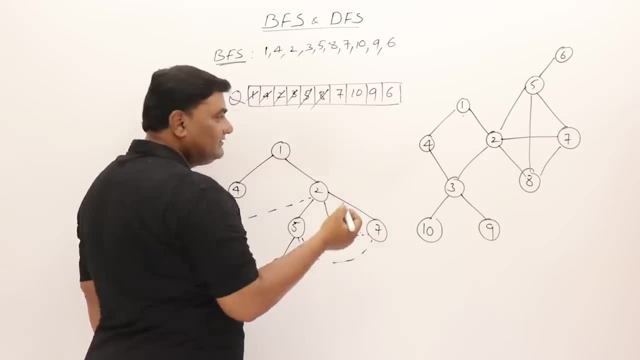 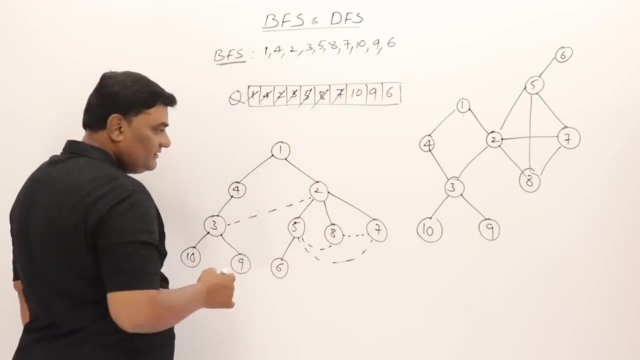 actually we came from there. seven draw a dotted line. so vertex which is already visited, we are drawing a dotted line. the next vertex for exploration: seven, seven is already explored. so is there anything remaining for seven? no, ten, there is nothing nearer to ten. no, nothing adjacent to ten. there is nothing as 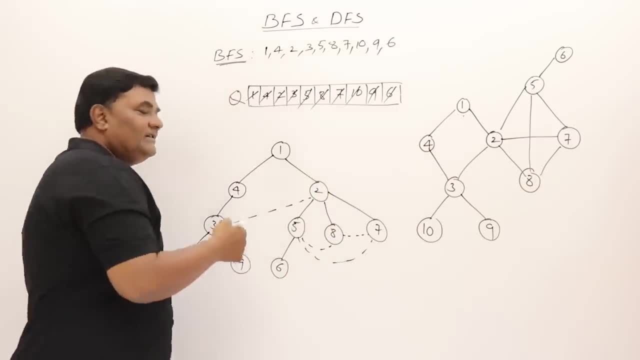 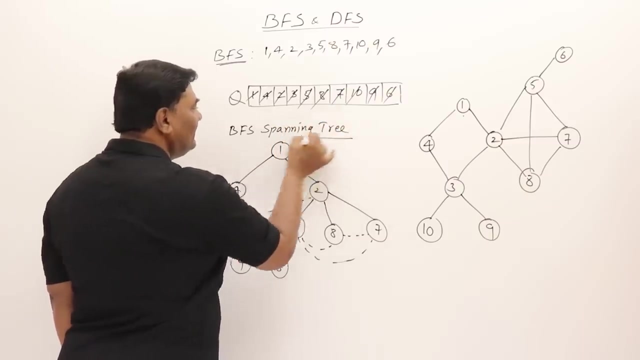 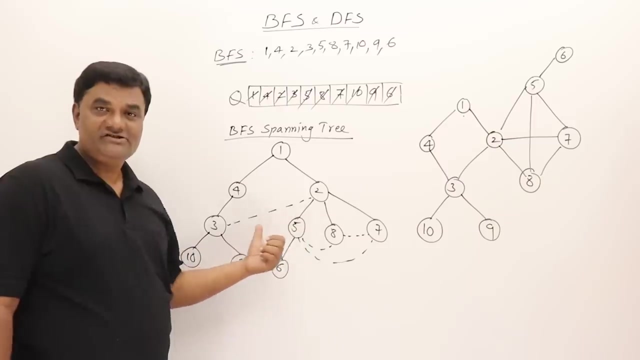 adjacent to nine and there is nothing adjacent to six. so that's all. this is breadth first search completed and the that we got here is breadth first search spanning tree dotted edges that we got here. they are called as cross edges. they are called as cross edges. let us see what. 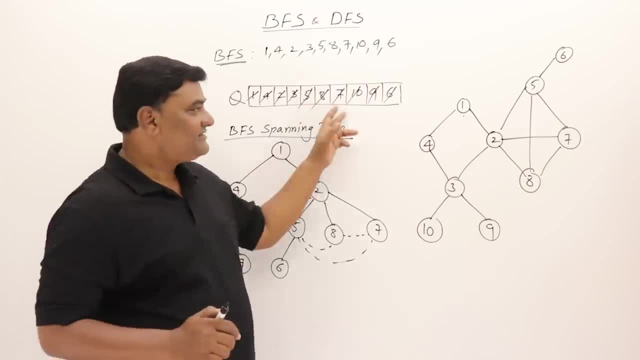 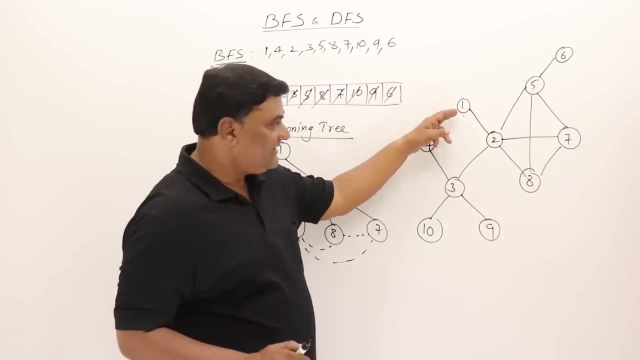 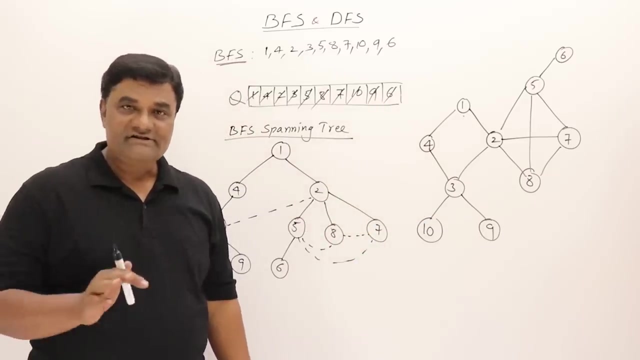 are the things that we have learned. first thing is you can start breadth first search from anywhere. next you like, first point. second thing is when you are exploring any vertex 1. Then you can visit this adjacent vertices in any order you like. This was the second thing. 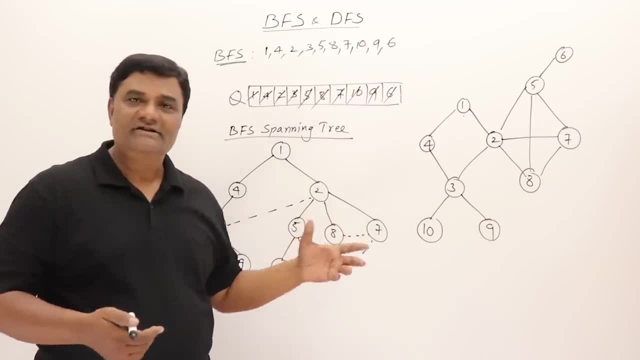 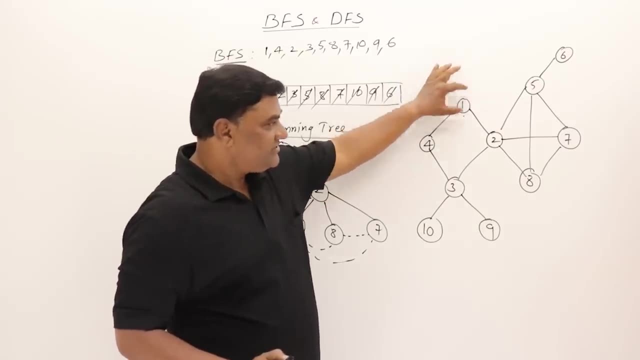 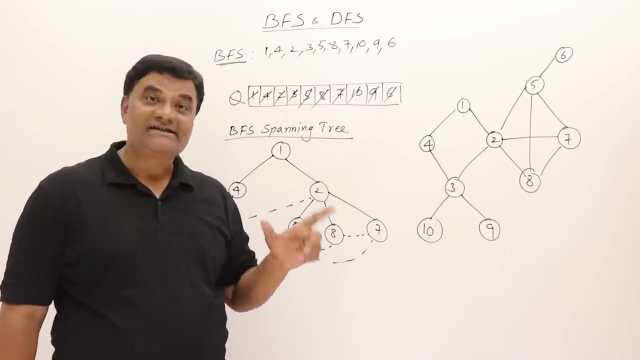 Then both are. leniency is given, freedom is given to select any vertex. Then what is the rule here? Rule is, when you are selecting a vertex for exploration, you must visit all its adjacent vertices. Then only you should go to next vertex for exploration. 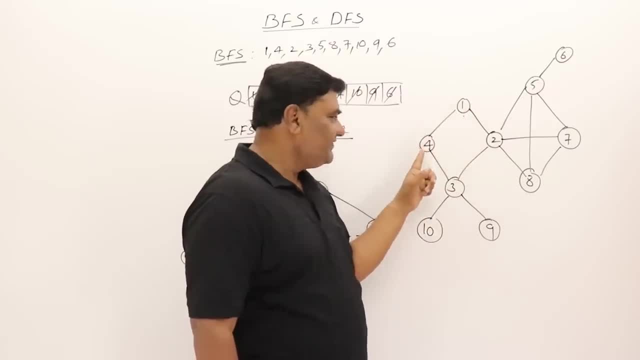 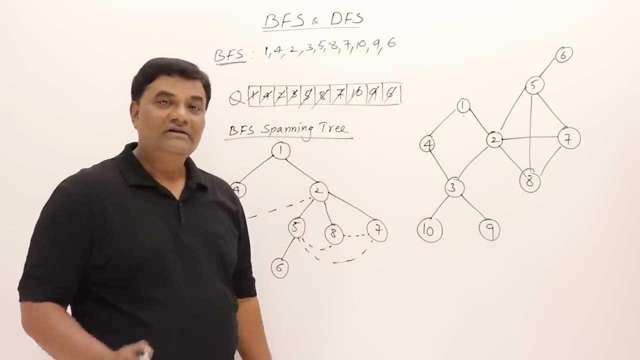 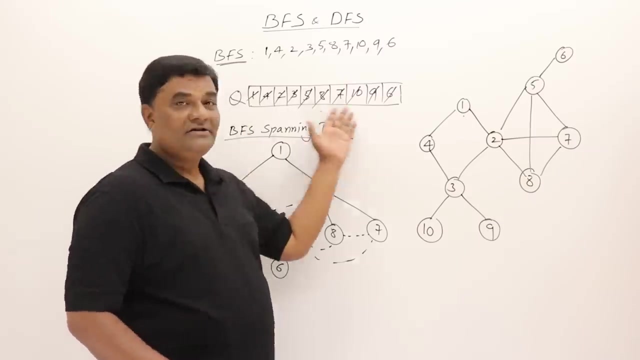 So if I am exploring 1, then I should visit 4 as well as 2.. Then only I should select 4 for exploration. This is the rule. The next thing is. last thing is, you should select the next vertex for exploration from a queue only. 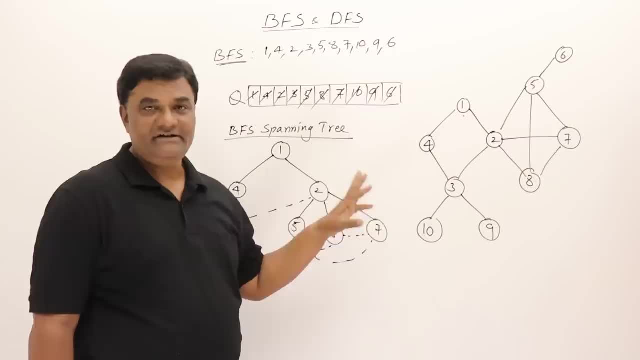 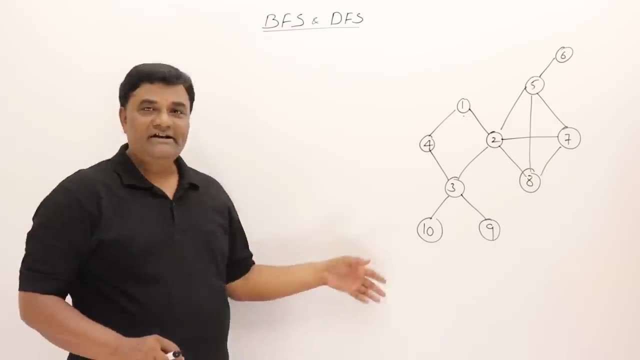 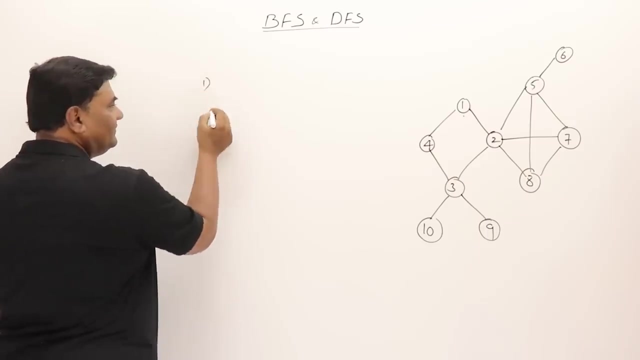 So queue and exploration should be completely done. These are the two important points about breadth first search. Follow this one then you can get many answers. I will write Few more valid breadth first searches here. First one: I will start from vertex 1.. 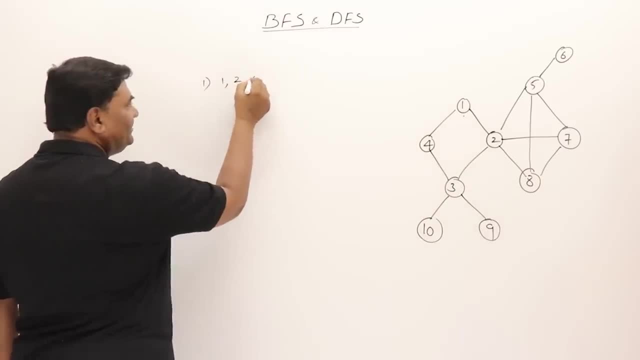 Then I will explore the adjacent vertices. So first I will explore 2, then 4.. Then I have to start exploring 2, because I have visited 2 first. So who are adjacent to 2?? So I will take 8, then 5, then 7, then 3.. 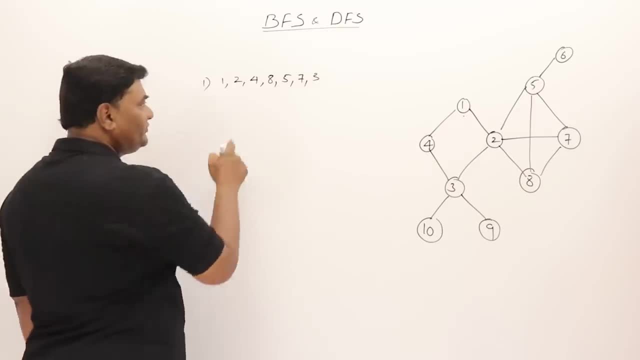 These are adjacent to 2.. All these are adjacent to 2.. Then I should explore which one: 4.. So who are adjacent to 4?, 4, 3. It's already over, Then explore 8.. Who is adjacent to 8?? 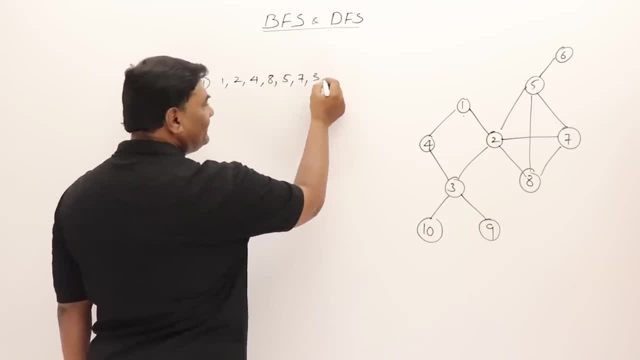 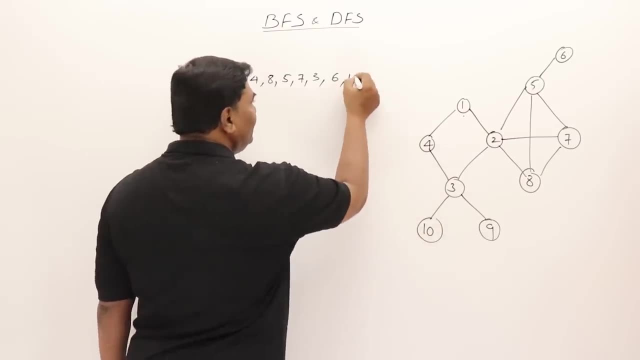 5 and 7. both are visited. Now explore 7.. So this is 6.. Now explore 3.. So 10 and 9.. So 10 and 9.. This is one also. This one is also a valid answer. 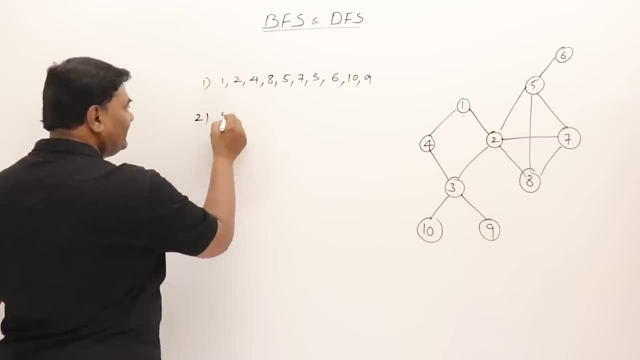 Then one more. I will start exploration from 5.. From 5, who are adjacent to 8,, 7 and 6? Now explore 8.. Who are adjacent to 2?, 3 and 1.. Now explore 8.. 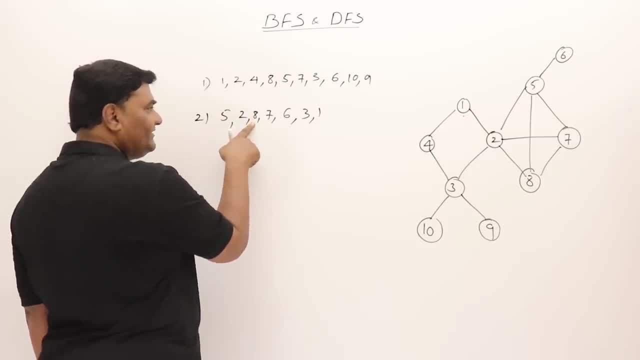 7 is already visited. 7. Everything is visited. 6. Nothing is there, So everything is visited: Explore: 3.. So 9 and 10. And 4. So for 3,, 9,, 10 and 4, I have visited. 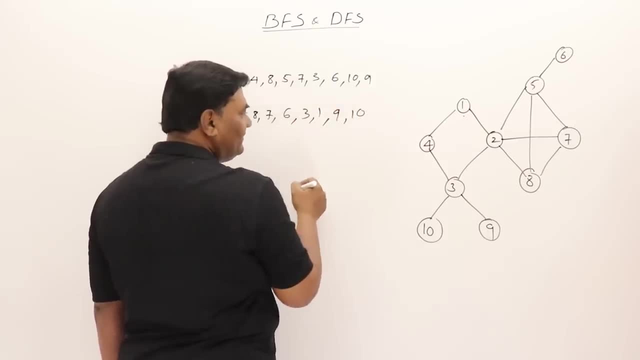 Now explore 1. Nothing is remaining. 9,, 10,, 4. All are visited, So this is also valid. So like this, you can start exploring. Explore 2.. Who are adjacent to 2?, 3 and 1.. 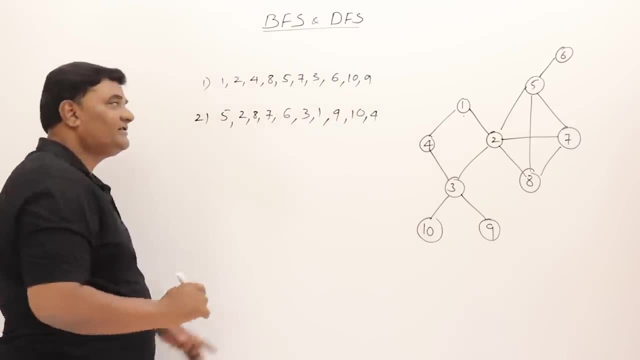 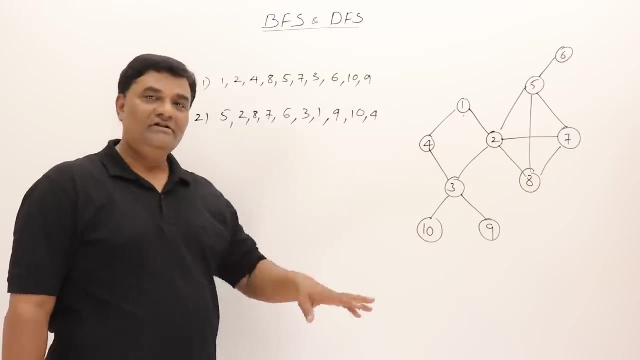 Now explore 8. 7 is already visited. 7. Everything is visited. 6. Nothing is there. So like this, you can start from any vertex and you can visit the adjacent in any order, So you can form numerous number of valid breadth. first search: 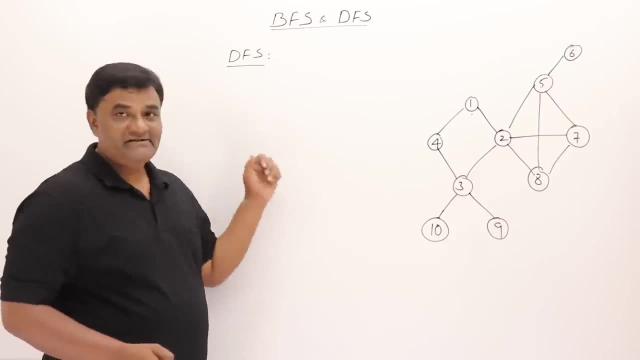 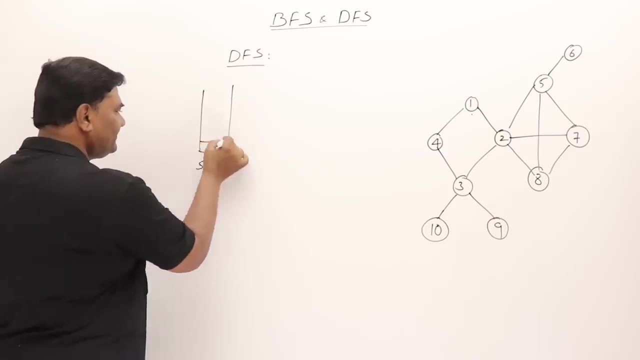 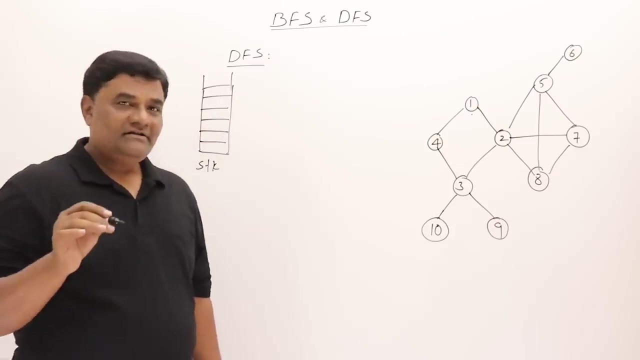 Next we will see depth first search. Now, next is depth first search. For this I will take a stack. Stack is a data structure used here. Let us start. I can start the traversal from any vertex. Start the traversal from any vertex I like. 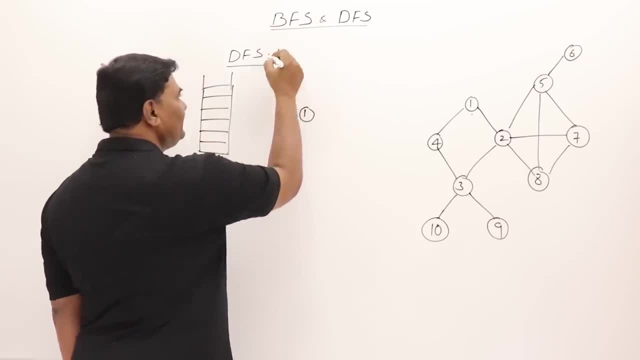 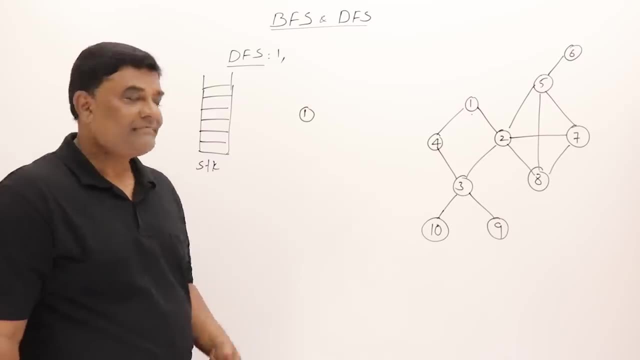 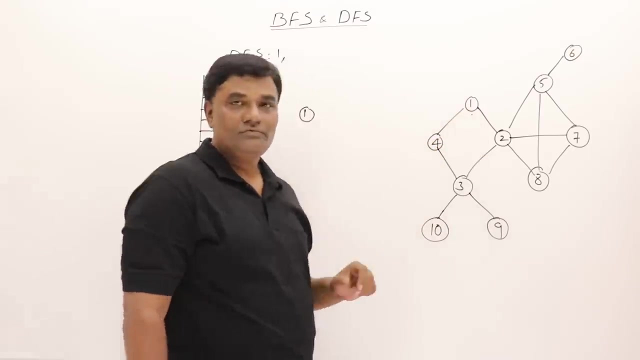 So I want to start from vertex 1.. So 1 is visited. This is the initial step. Now the repeating step. What I have to do every time As this new vertex is visited: start exploring it. So who are adjacent to that 4 and 2?? 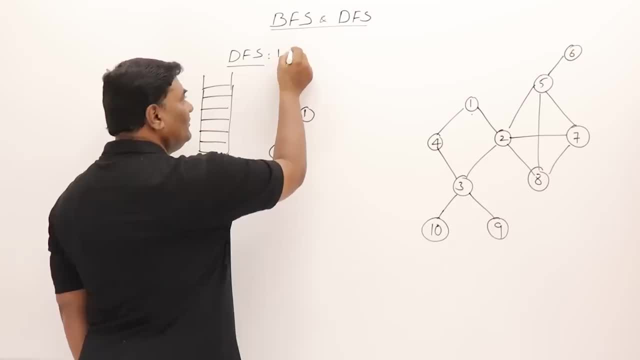 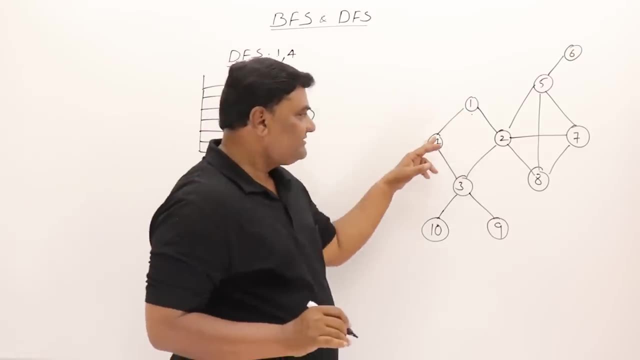 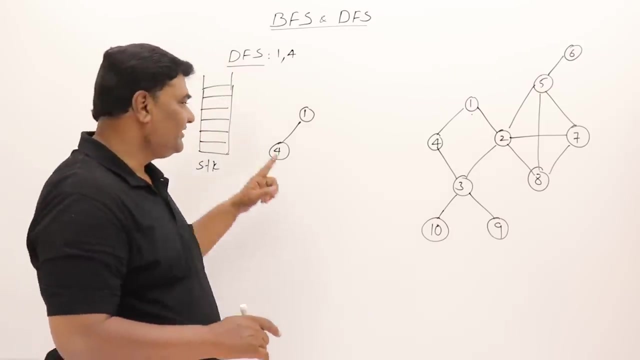 So visit 4,, 4,, 4.. Now the rule in depth first search is depth, first searches. once you have visited one vertex, still one more is remaining. leave that we will see it afterwards. first you start exploring four. so this is the rule. so once. 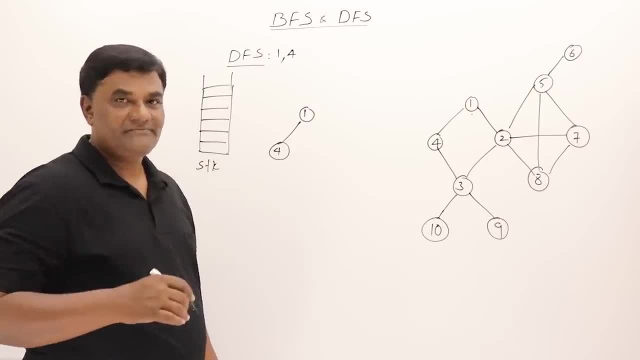 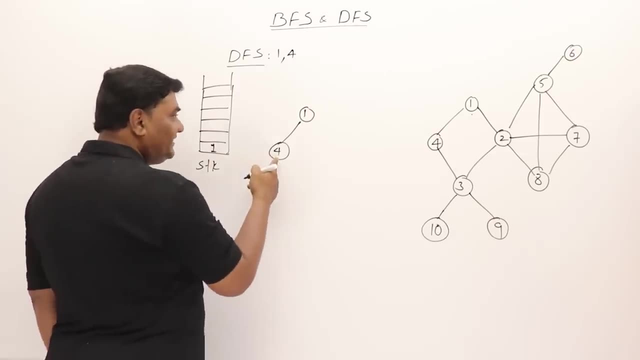 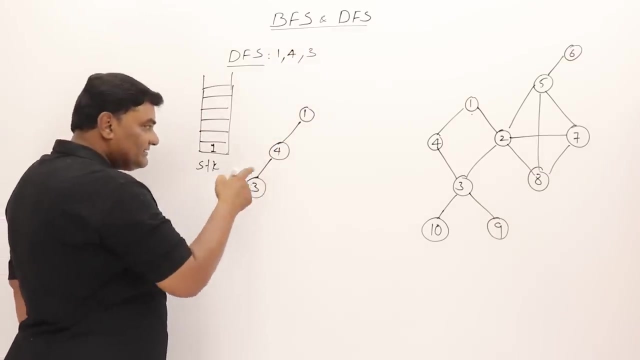 you have reached a new vertex, start exploring that new vertex. what about that one? suspend it and keep it in the step that we can explore it later. now start exploring four. so from four i can go on three. so okay, go to three. three is visited. now what to do? suspend four and start. 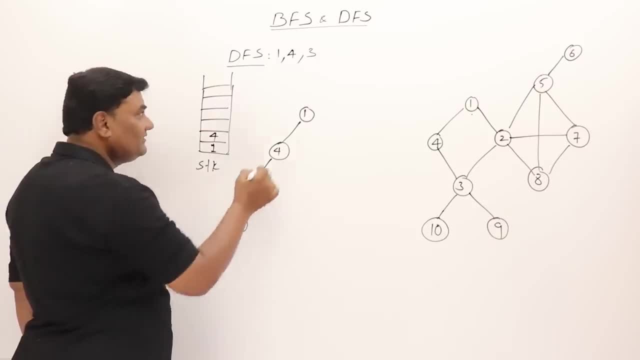 exploring three. from three i can go on ten. so ten. suspend three, start exploring ten. there is no adjacent vertex of ten, so go back to three. so how to know i where i have to go back? this stack will give me their value. so this three continue exploring three. so i can go on nine, nine and 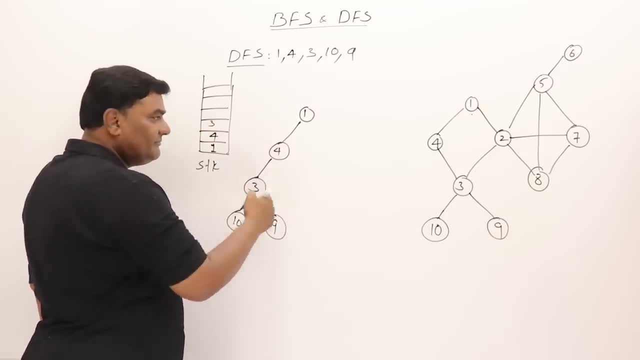 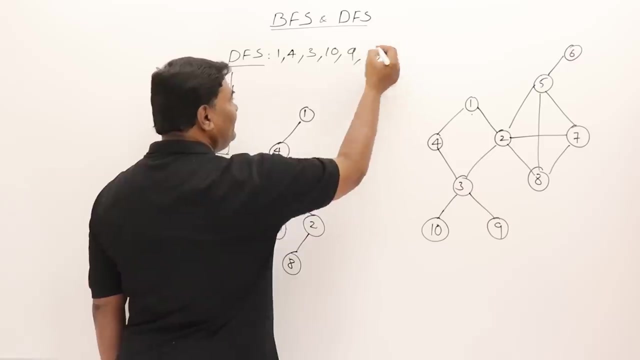 again, suspend three and start exploring nine. from nine, i cannot go anywhere. then go back to three and start exploring three. so who is adjacent to three? two, so two is visited. then from two, who is adjacent, suspend two and start exploring two. so from two, eight is adjacent. so take eight, now start. 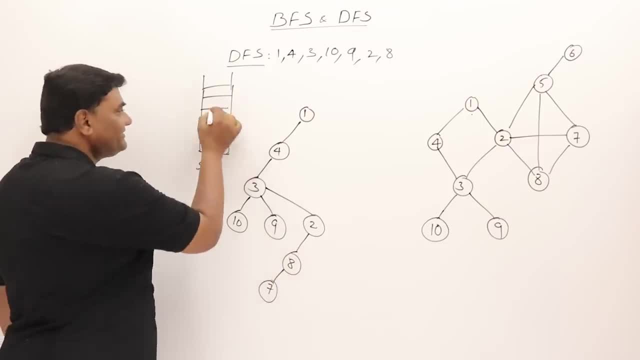 exploring eight. so from there i can go on seven. so suspend eight. so seven is visited. now we have to explore seven. from seven i can go on five. so five is newly visited. now we have to start exploring five. so suspend seven and push it into the stack. 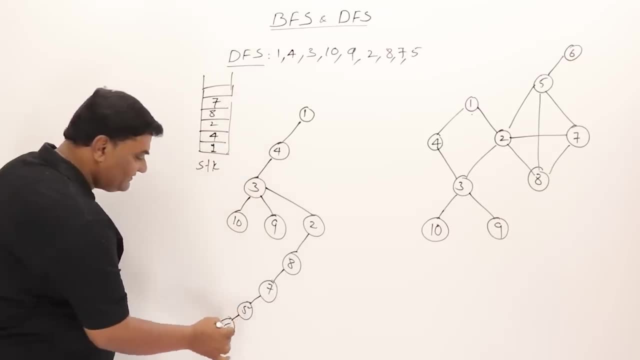 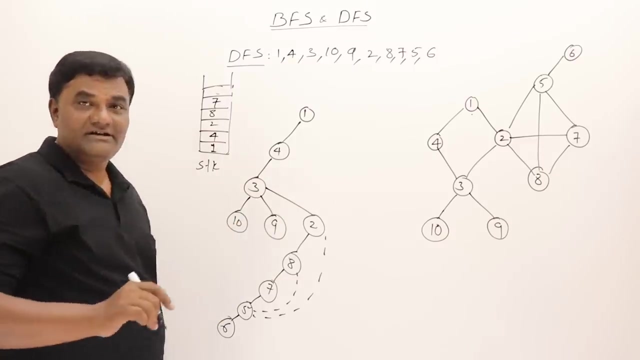 then, from five, who is adjacent six, so visit six, suspend five and continue exploration of six. there is nothing adjacent to six, so go back to five. from five, where i can go further, so i can visit two, which is already completed. right, i can visit eight, which is already completed, so there is nothing remaining for five. so what happens in this way is we are 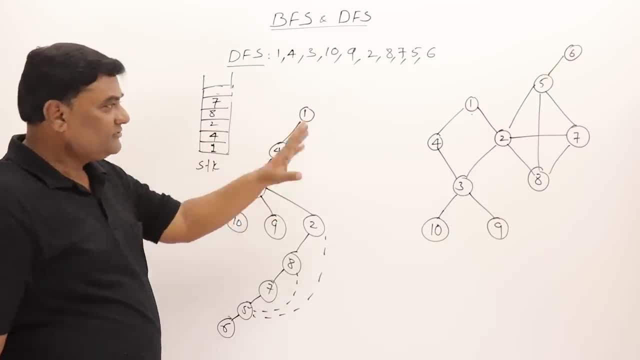 going deep and deep right. so in this way, almost all vertices are visited, only they are completely explored. so five is completely explored. go back to the previous vertex. who is that? seven, seven from seven, where i can go from seven. i can go on two, which is already visited. 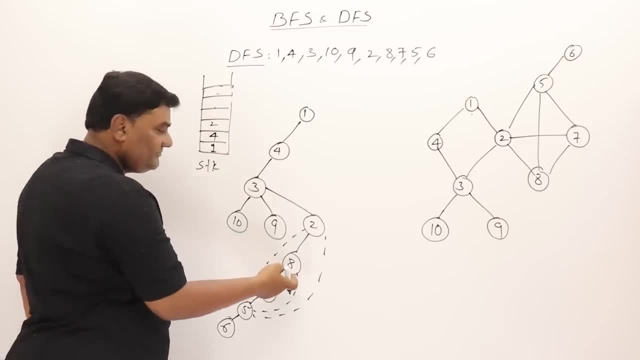 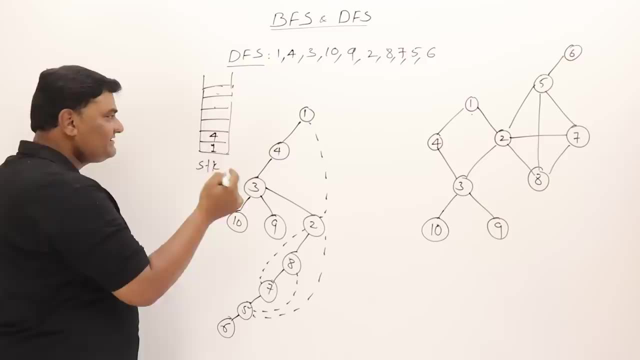 then go back to eight. from eight, nothing is remaining so from two, where i can go, i can go to one, right then nothing is remaining. so go back to four. from four, i cannot go anywhere. from three, one, i cannot visit anywhere. so that's all right. so here is the defer search traversal result. 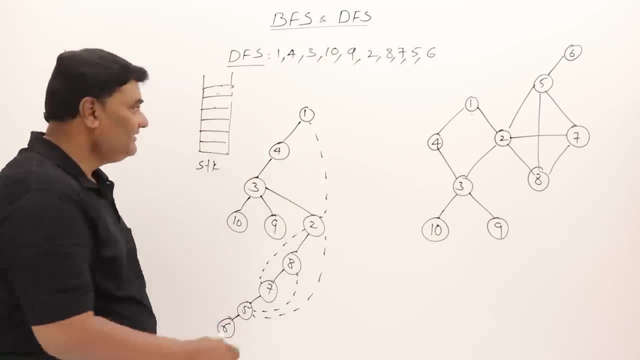 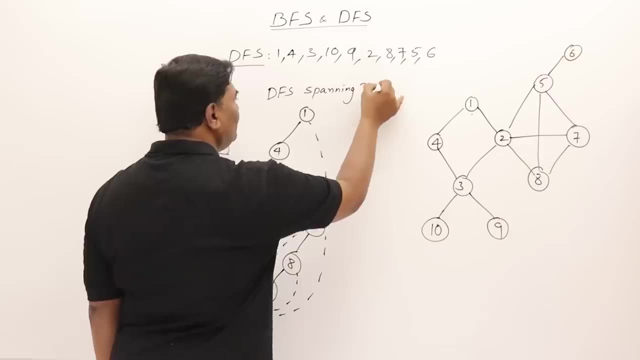 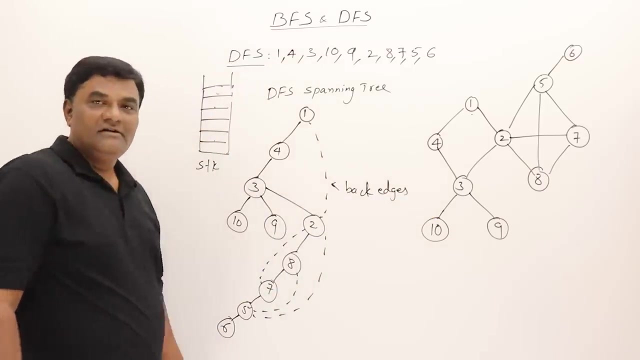 and this is a dfs spanning tree. this is depth four search spanning tree and these edges are called as back edges. so for this graph we can make a tree like and perform pre-order. so this is the pre-order of this tree: see one, four, three, ten, then nine, then two, eight, seven, five, six.